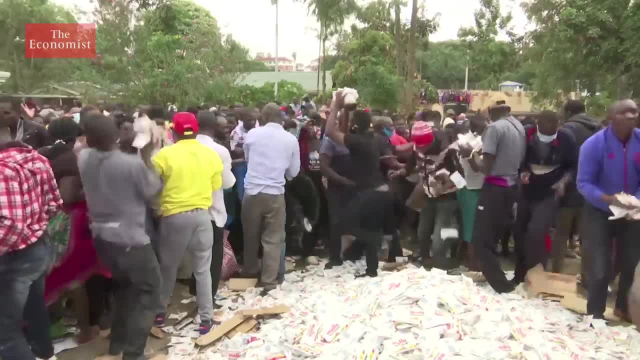 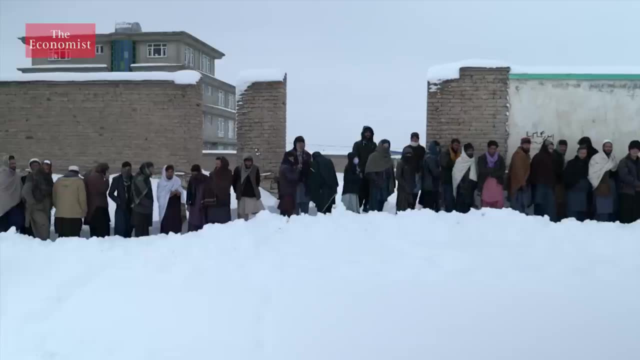 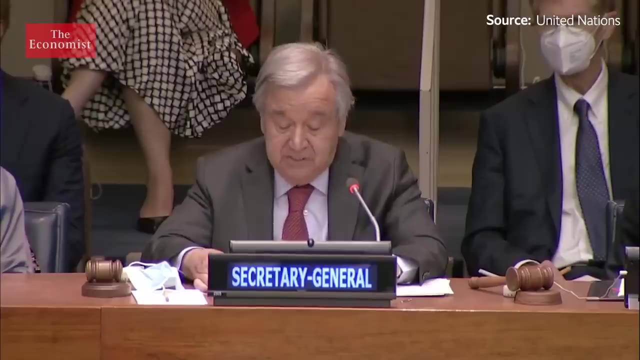 An unprecedented food crisis is engulfing the world. supercharged by the war in Ukraine, It's brought rising food prices, malnutrition and the potential for much, much worse. It threatens to tip tens of millions of people over the edge into mass hunger and famine. 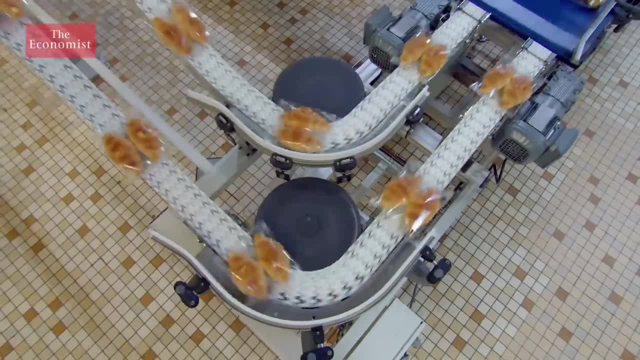 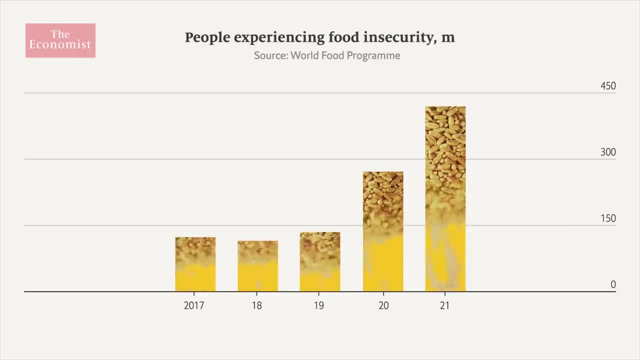 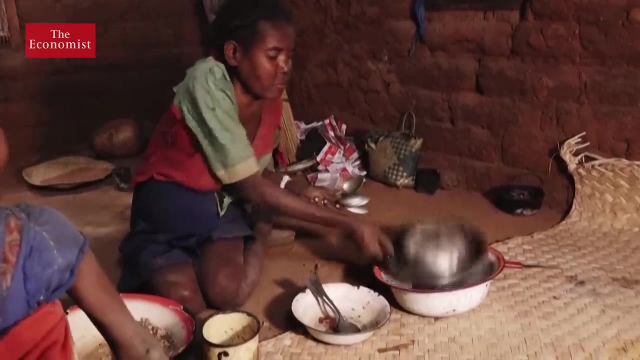 Until recently, global hunger was in decline, But since 2014, it's been rising. Over the past two years, the number of people without regular access to food has more than doubled. Some 800 million people already go to bed hungry every night. 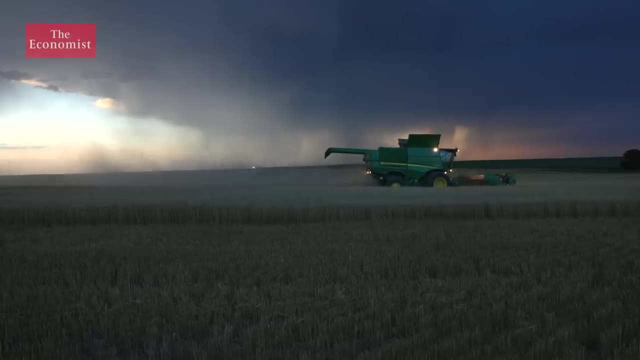 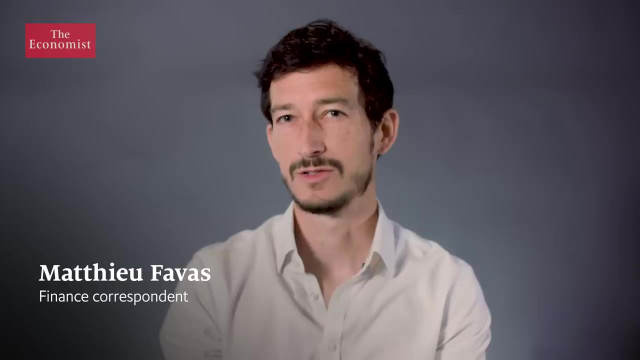 And now the world's food system has been hit with a perfect storm. 2022 was already looking like a terrorist attack. It's a terrible year for global hunger, as COVID still continues to grip some parts of the food supply chain worldwide. 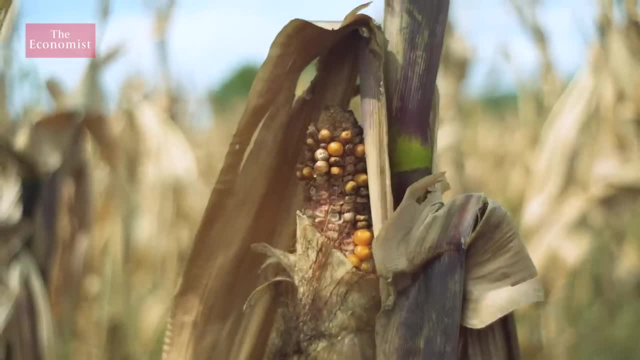 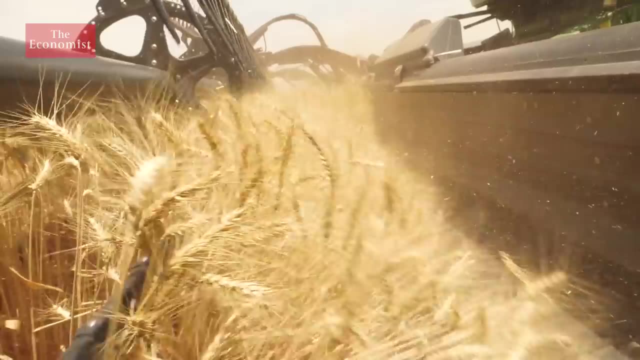 You've had a series of bad harvests in recent years because of climate change. This all disrupted food production. Those two shocks- climate change and the pandemic- have meant that, according to one estimate, global supply of wheat- one of the world's most important carbohydrates- 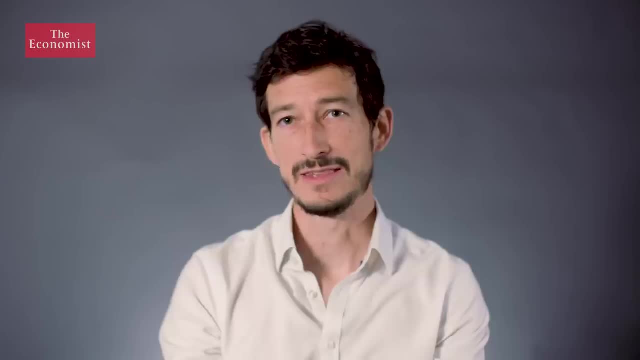 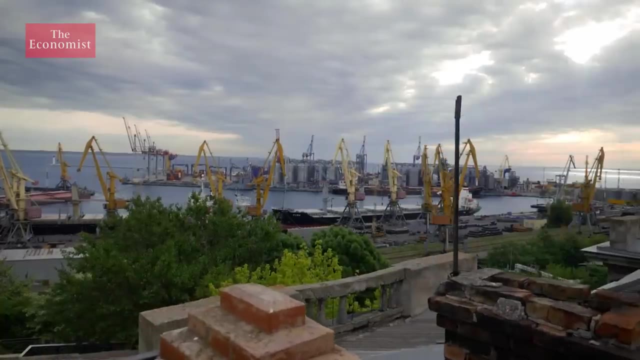 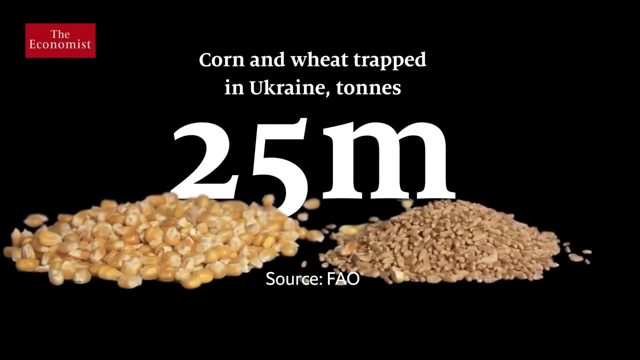 has fallen for the first time in four years. And then the war happened. Ukraine's food exports all but stopped, Trapping around 25 million tonnes of corn and wheat inside the country, Equivalent to the annual consumption of all of the world's least developed economies. 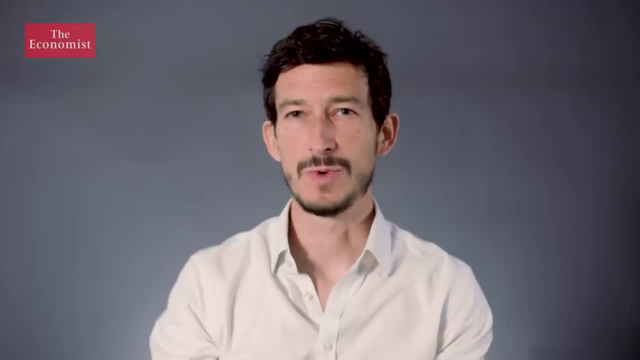 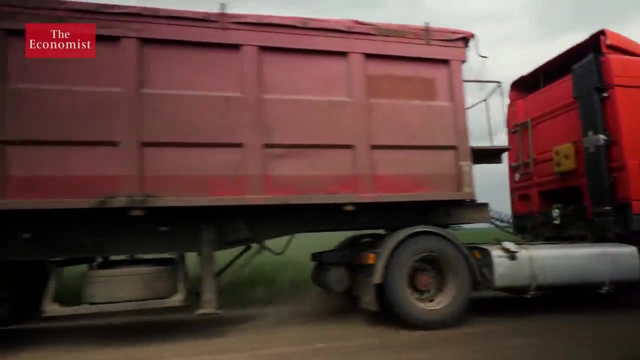 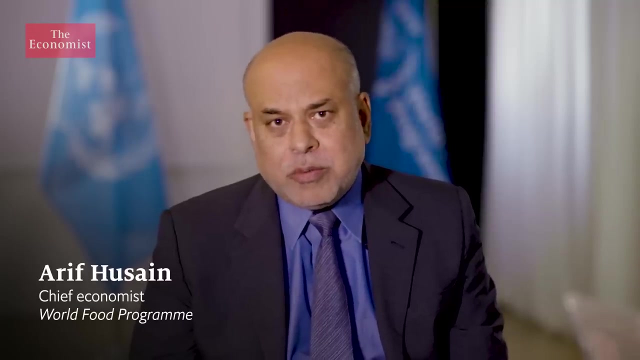 Ukraine's food exports are hugely important to the global food supply. It's a big powerhouse in terms of grain production. It's one of the world's breadbaskets And with that breadbasket off the market, prices rocketed. Imagine if you were buying your food from Ukraine. 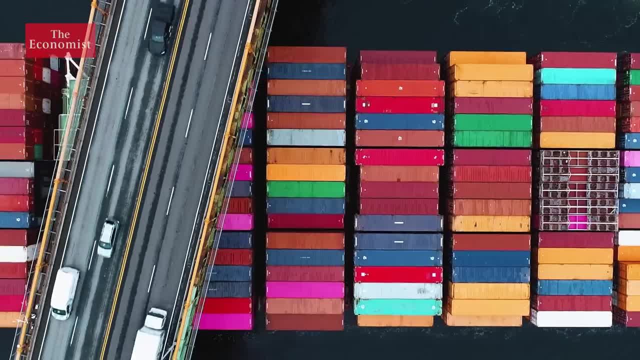 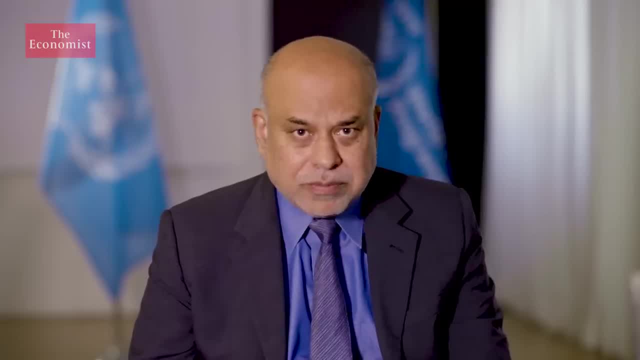 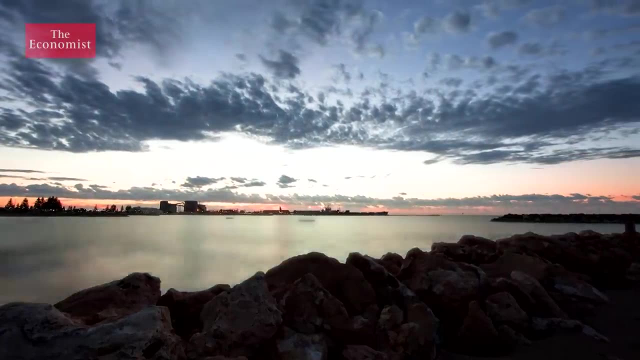 And now let's say you need to go to Canada or Australia or Argentina. That means that you will have to pay more because of extra freight And you will have to pay more in time because it will take you longer And you will pass these costs to the consumer. 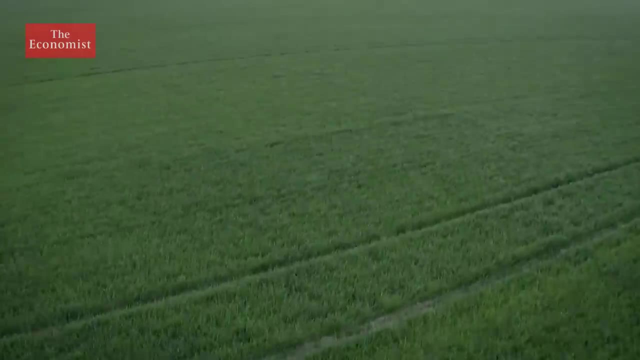 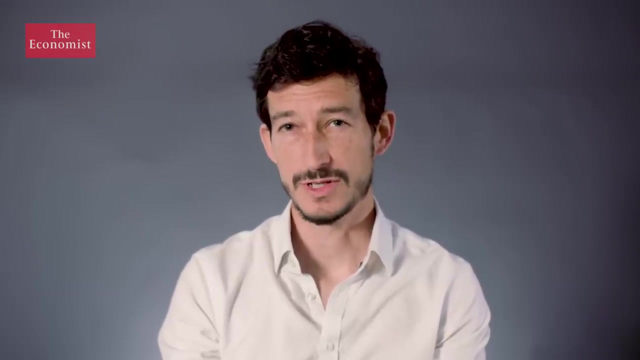 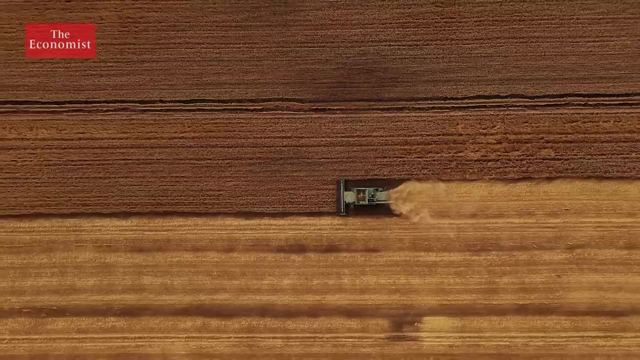 And other shocks have made the crisis worse. We are in uncharted territory because not only do we have a food crisis with multiple causes, but also this is coming on top of an energy crisis and also a fertilizer crisis. Farms run on fuel and fertilizer. 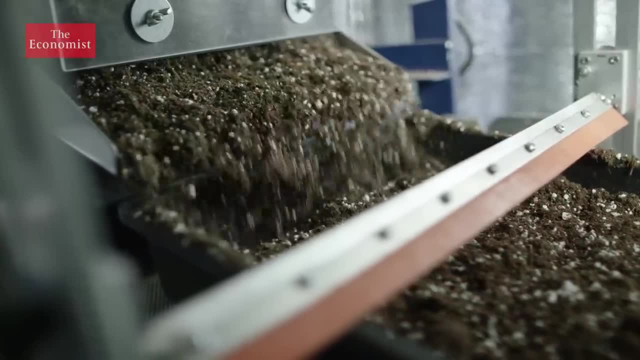 As prices of both have risen, farmers' profit margins have been squeezed, And if they're forced to cut back on fertilizer because it's too expensive, Farms run on fuel and fertilizer. As prices of both have risen, farmers' profit margins have been squeezed, And if they're forced to cut back on fertilizer because it's too expensive, 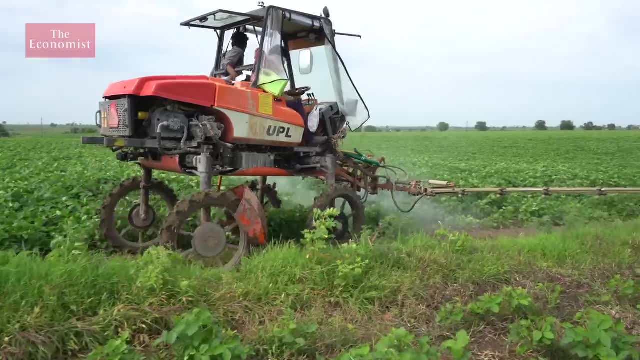 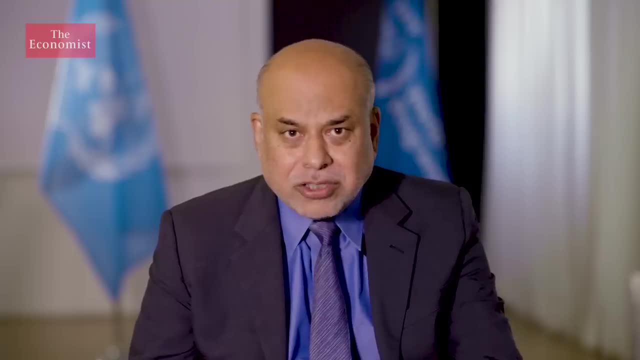 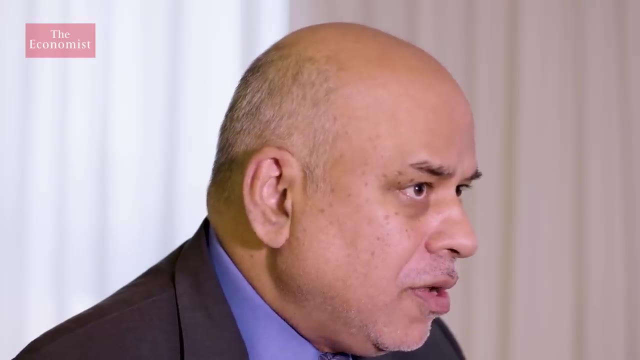 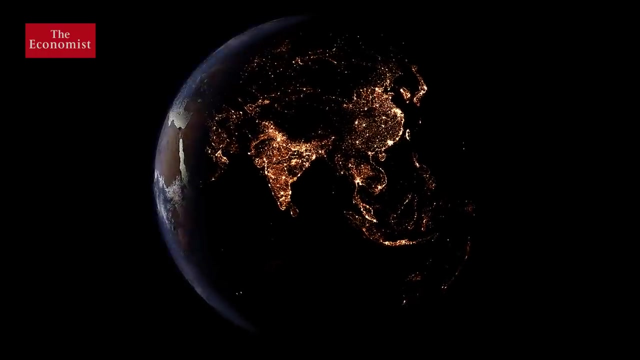 or unavailable, their yields will fall even more at the worst possible time. That will impact the production of major commodities for the next year. And then we are looking at an availability crisis. Imagine what that would do to food prices. It's a vicious cycle with potentially catastrophic consequences. 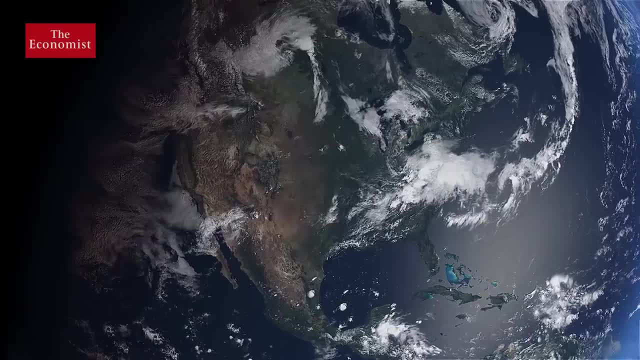 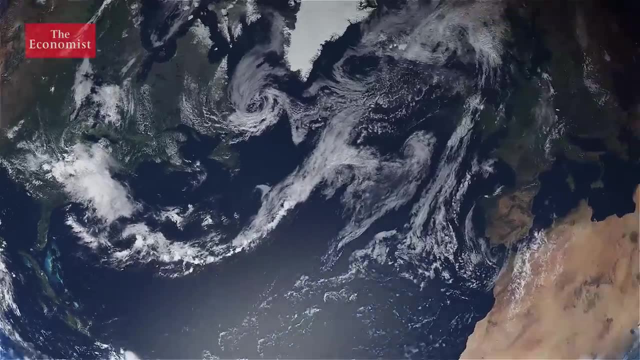 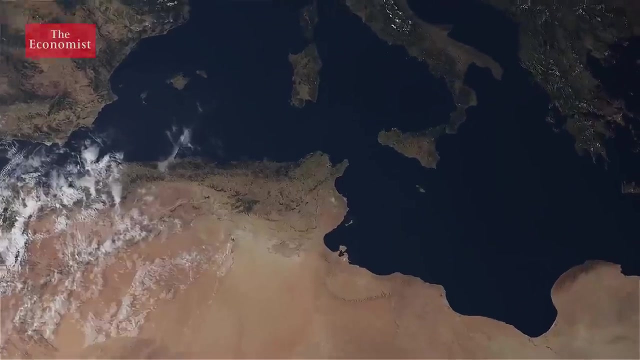 And no doubt nowhere on earth is immune. In America, rising food and energy costs have helped push inflation to its highest levels since 1981.. Food prices in Britain are rising at a rate not seen for 13 years, And in poorer countries things are even worse. 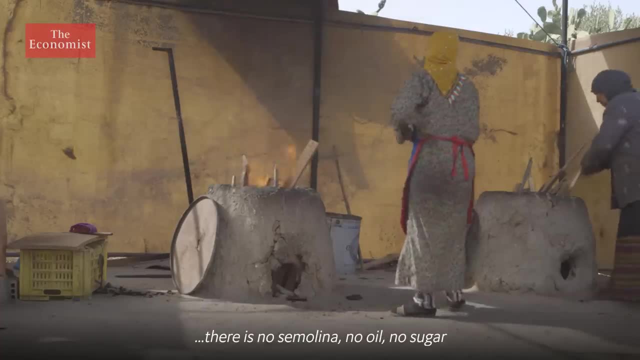 I'm hungry, I'm starving. I don't have any food, no oil, no sugar. If I take a drop of oil, they'll tell me I didn't take it. If I take a drop of oil, they'll tell me I didn't take it. 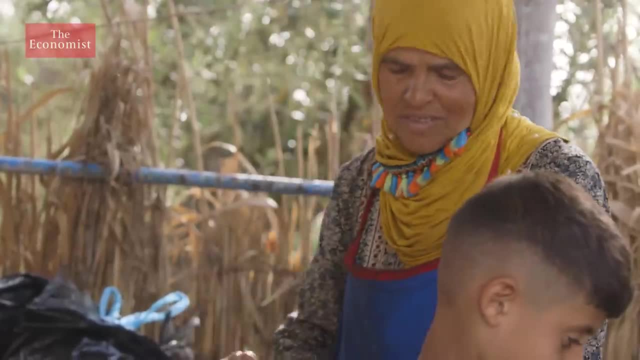 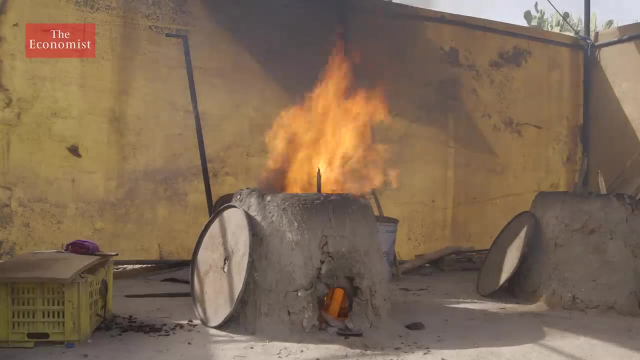 If I take a drop of oil, they'll tell me I didn't take it For Souad, the food crisis has already hit home. She's been selling Hobstabouna, a traditional Tunisian bread made with semolina, for the last 35 years. 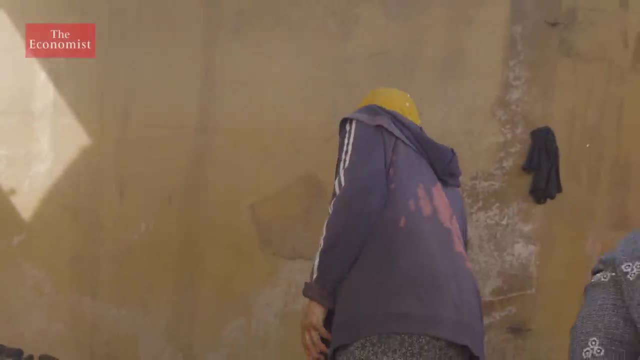 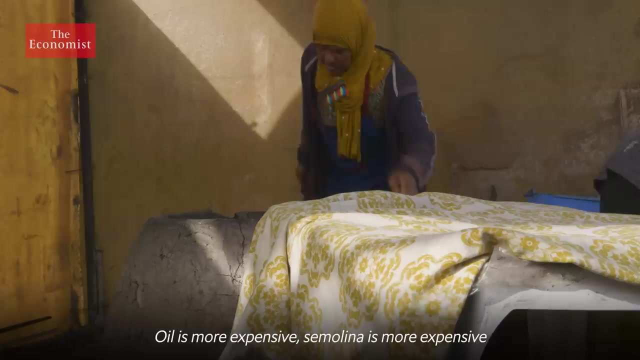 Now the cost of her ingredients are going up and customers are buying less, leaving her with less money to feed her family. It's hard to go. The oil is expensive. The semolina is expensive If you take five or six or two or three. 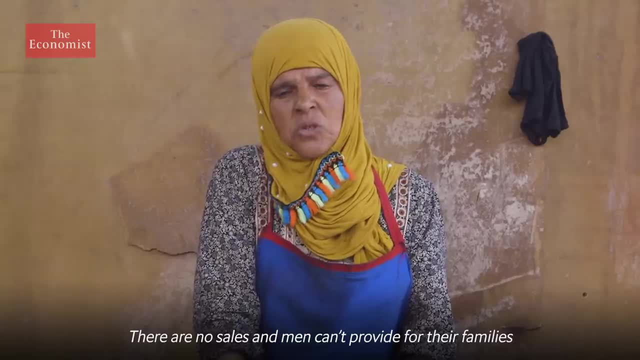 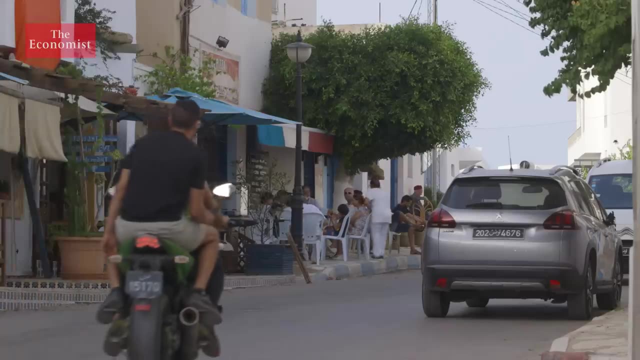 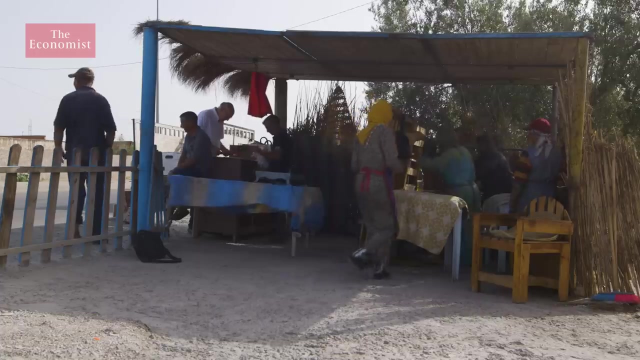 the semolina is only for the small ones and the big ones. Tunisia usually imports about 42% of its wheat from Ukraine and relies on it for sunflower oil, another crucial commodity. With those imports gone, Tunisia has struggled to find other suppliers it can afford. 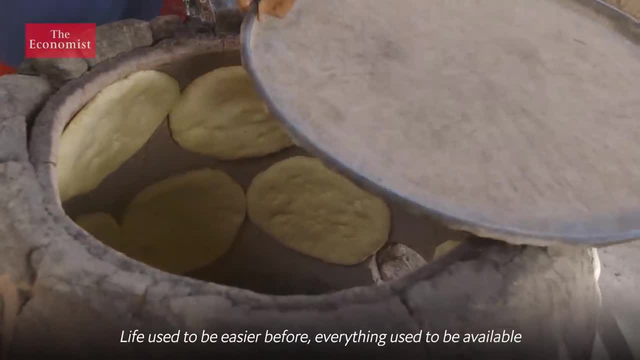 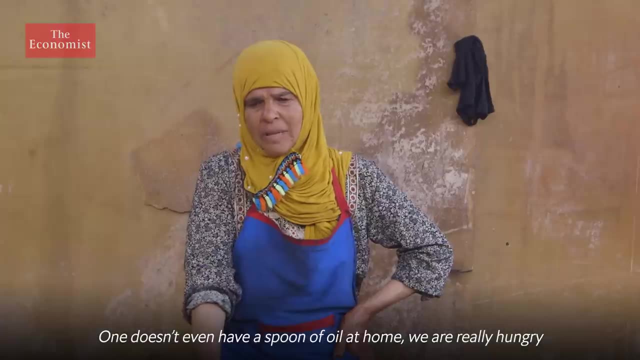 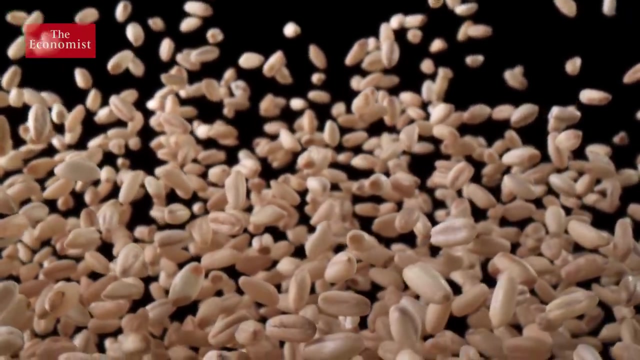 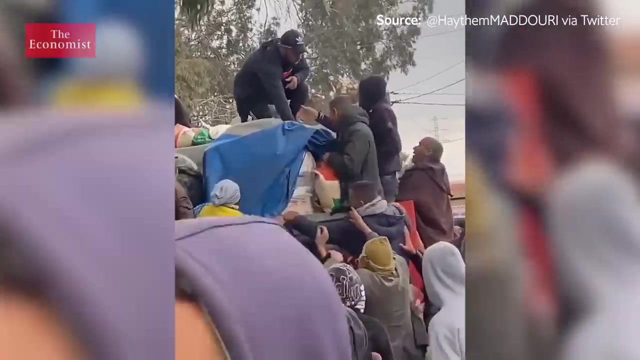 meaning shortages. for people like Souad, It's not easy. everything is better than it used to be. When you go into a house, it's a mess. In Tunisia, hunger is turning to anger As food disappears from shelves. there's a risk Tunisians could lose patience with their government. 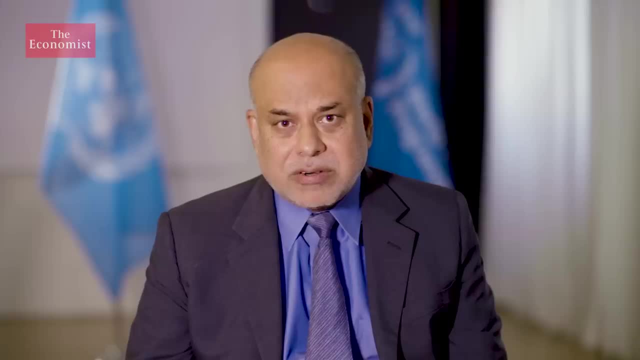 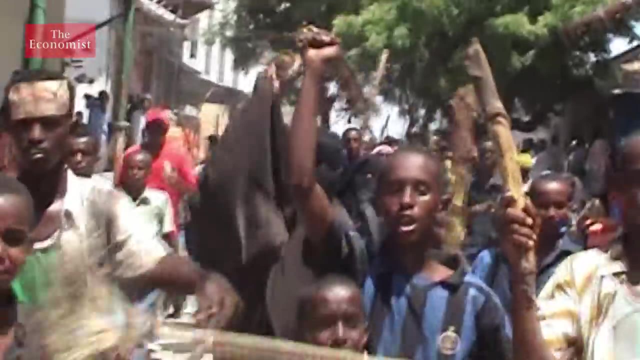 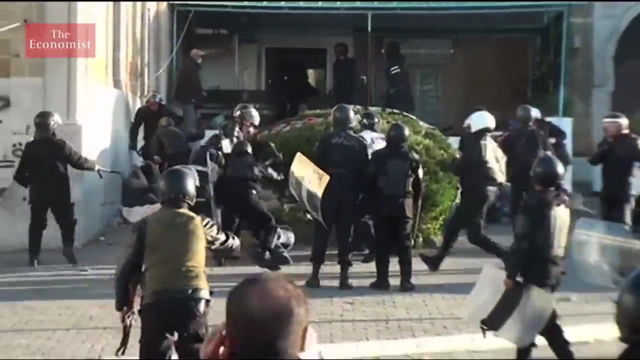 I'm really, really concerned about how this crisis can affect the economy, and I want the people of Tunisia to see that it's not just about money. it's about our people. We saw a lot of riots that broke civil unrest In 2008,. 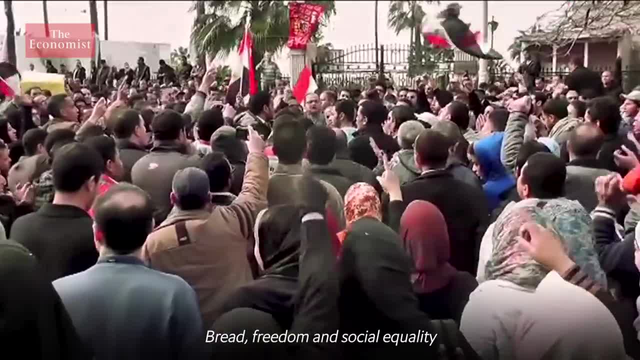 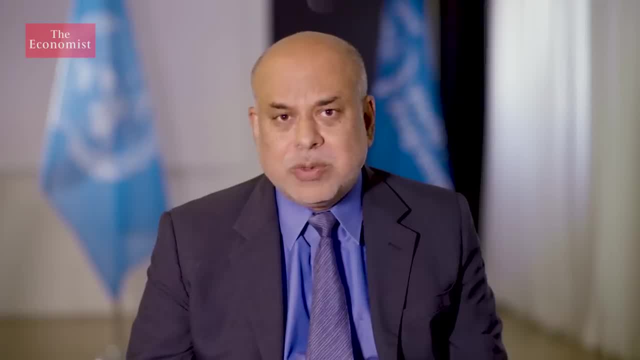 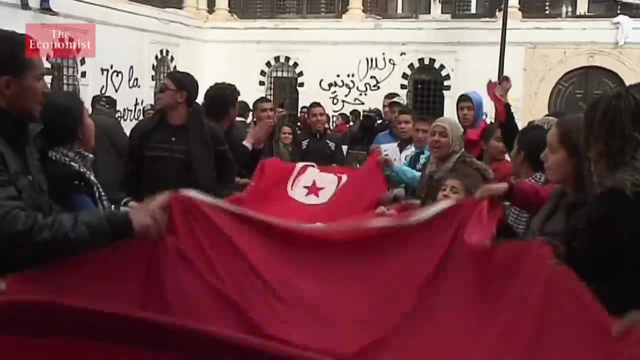 we saw riots in upwards of 40 countries In 2011,. we saw riots, but also the start of the Arab Spring. Today, we are looking at something which we haven't seen before: prices. some believe it was a contributing factor. 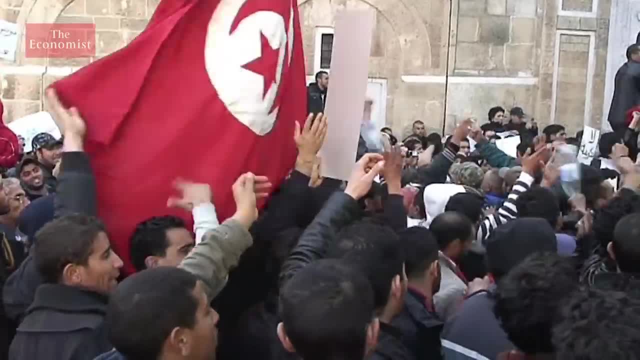 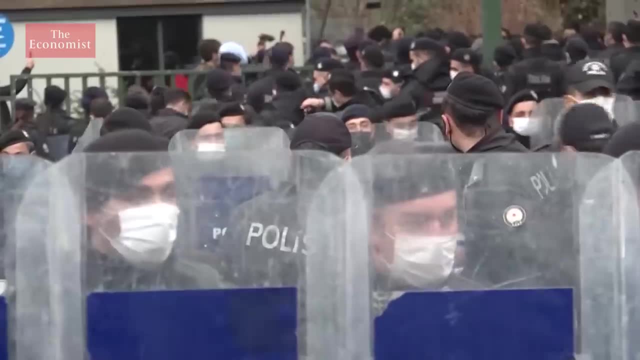 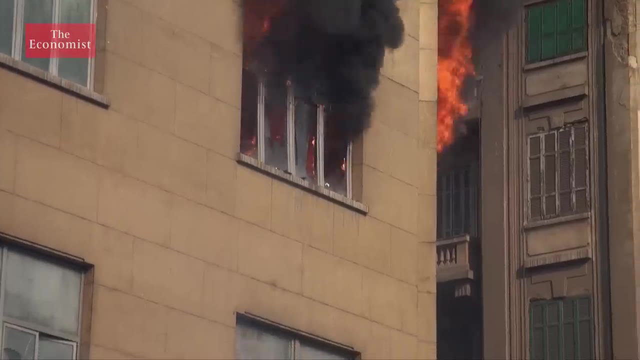 And it's not just in Tunisia, where hunger looks set to cause problems for governments. The economists' modeling suggests that many countries could see a doubling of the number of serious outbreaks of unrest over the next year, And it wouldn't just be anger driving this unrest. 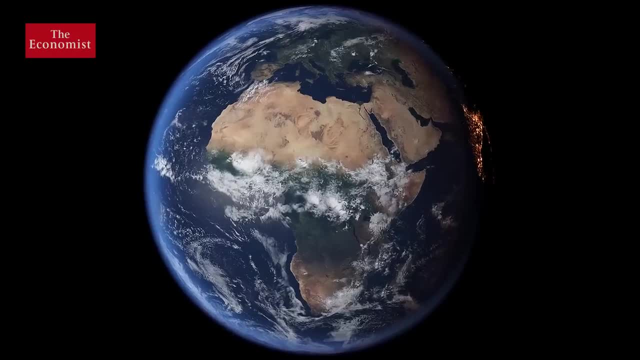 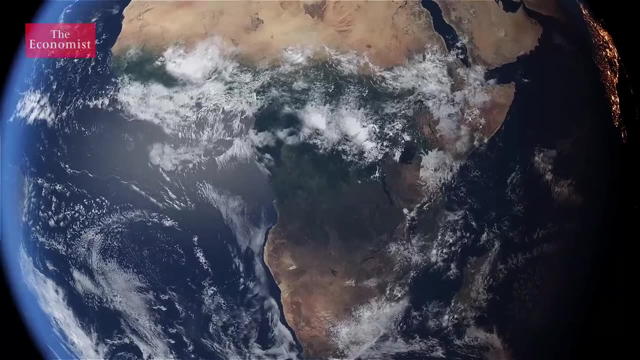 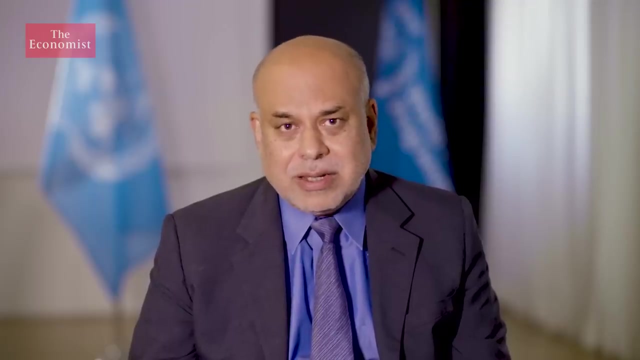 but a genuine fear of going hungry. Households in sub-Saharan Africa already spend up to 40% of their income feeding themselves. A rise in prices means millions won't be able to afford to eat. In many, many cases, their best day is like our worst day. 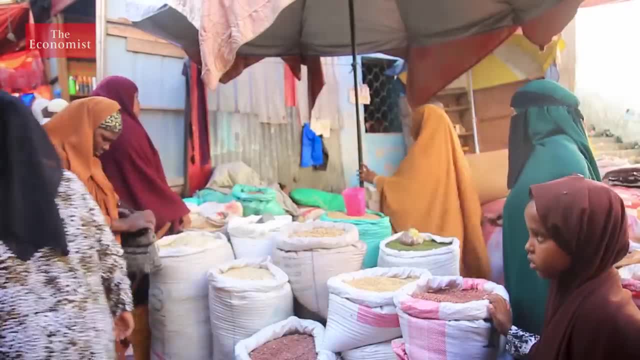 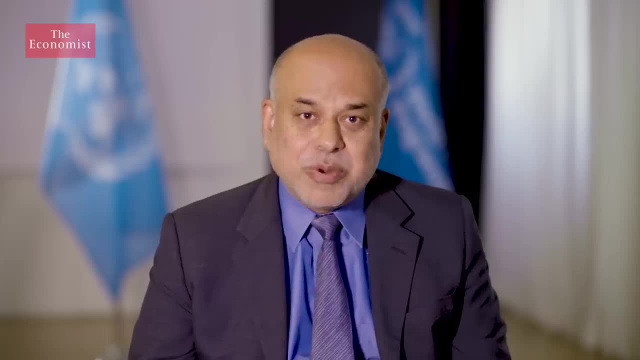 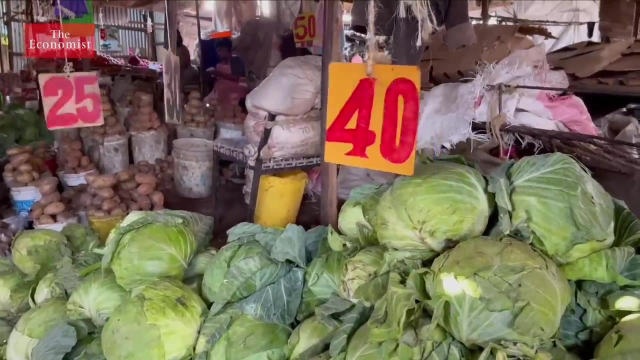 Imagine if you are spending 50% of your income just on food. How much space do you have for anything else? And then the prices of two things which really really matter, meaning your food and your fuel- they go up, Governments are tapped out. 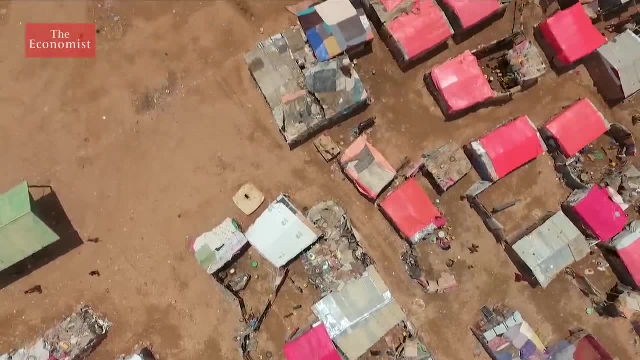 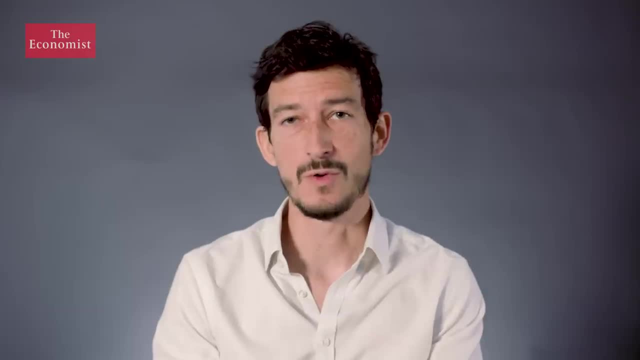 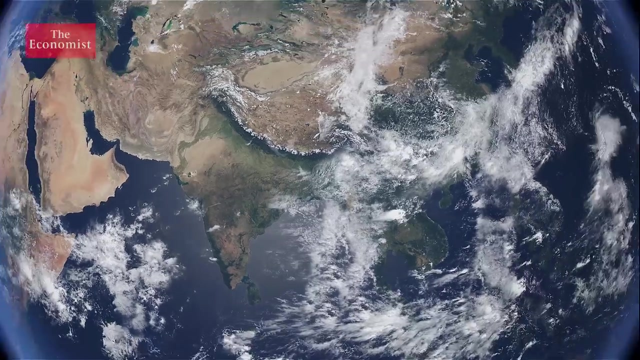 There are no safety nets. Those that do have supplies have been turning inwards. There are a number of fixes that countries are turning to. One of the unfortunate ones is protectionism, That is to say, export controls and stockpiling Following severe heat waves earlier this year. 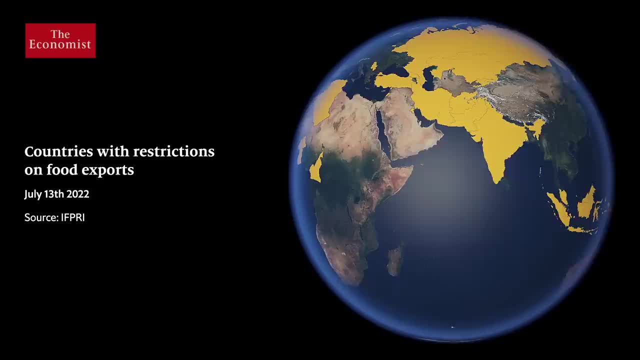 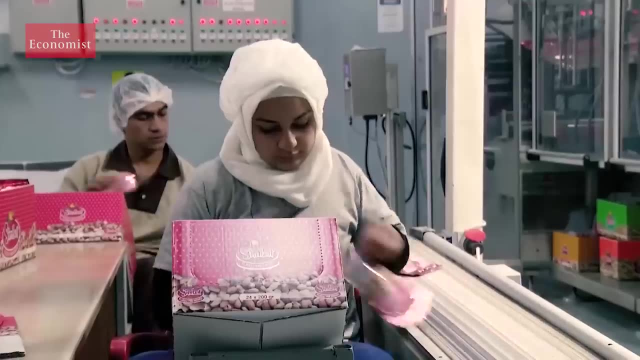 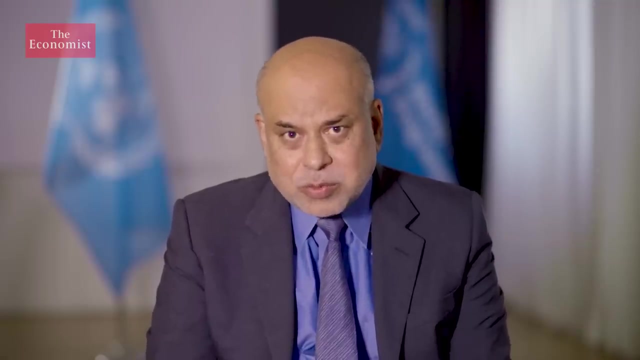 India banned wheat exports. In total, 23 countries now have severe restrictions on food exports. The thing is, they might be doing themselves more harm than good. Time and again it has been proven that it doesn't help inside the country which puts the export ban. it doesn't help outside the country. 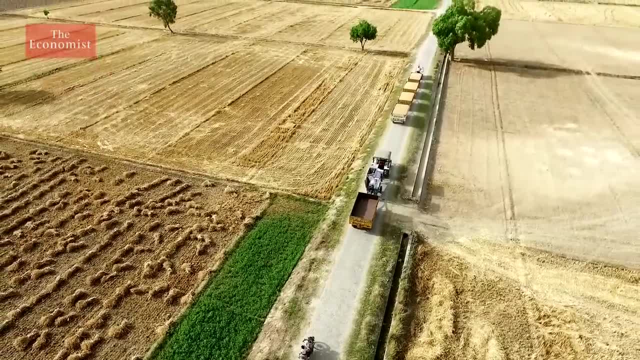 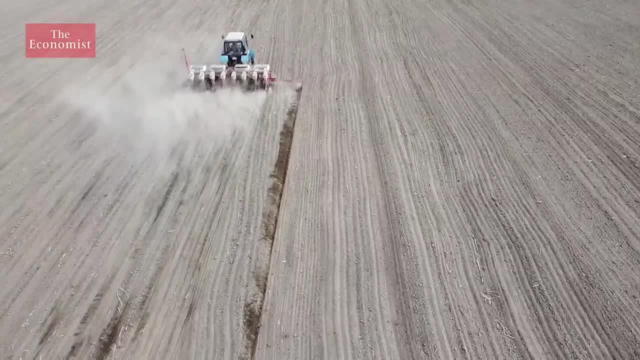 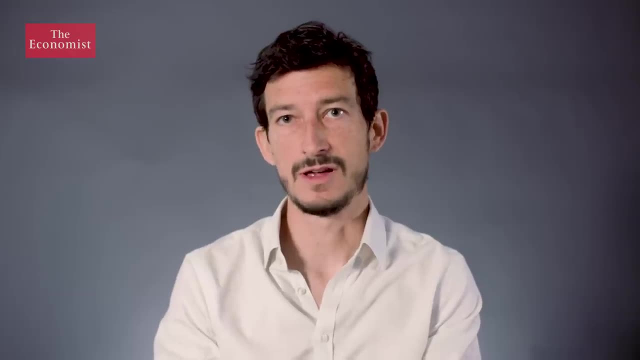 Export bans can make a price problem worse. Farmers may hoard their products until the ban is lifted, Or they might even switch to another crop. That would reduce domestic supply for food and push prices up. Whilst you can sympathise with these countries that are doing this, 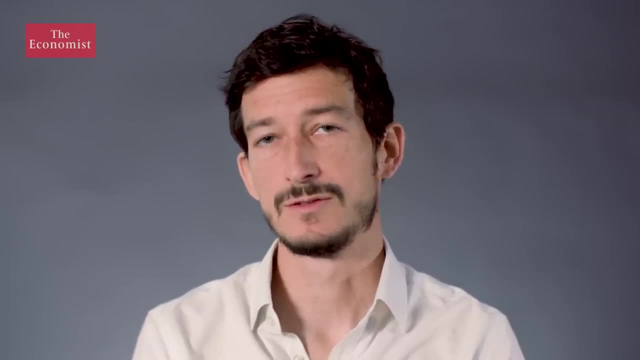 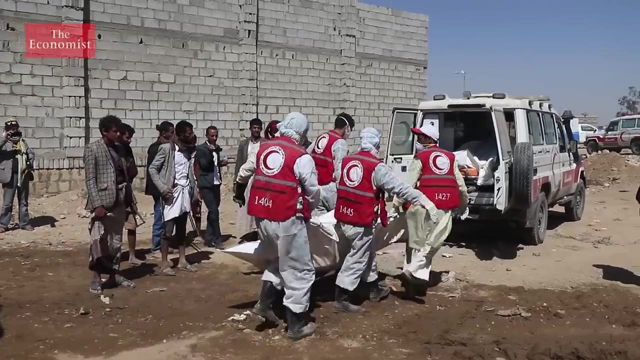 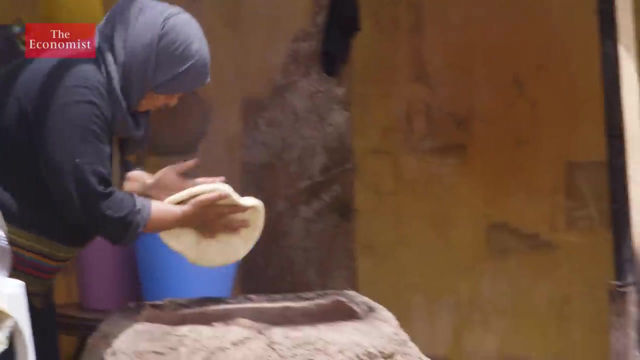 the result is potentially much higher prices for everyone else. That means the challenge faced by some of the world's poorest countries could grow even further. We need to help governments reach their populations with affordable food, with affordable fuel, with fertiliser, And what that will require is 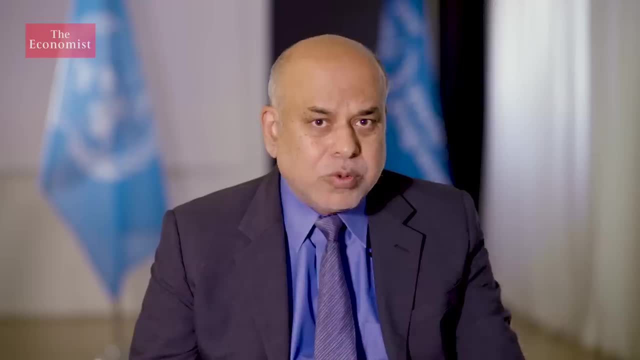 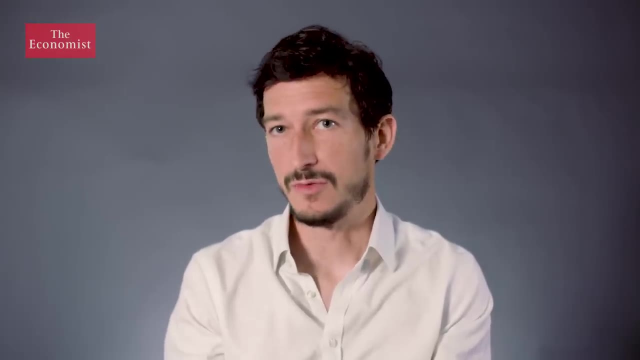 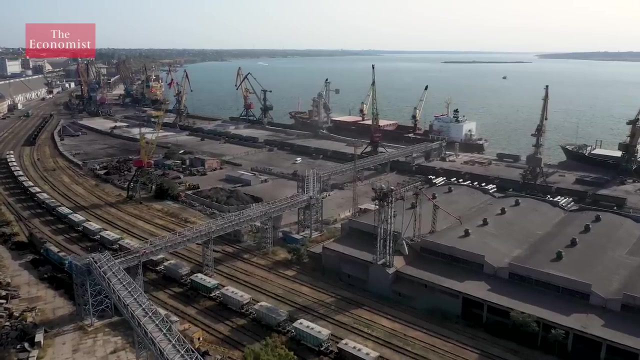 facilities, financing facilities which are accessible to these governments to do that, Providing some loans at a low rate, through the IMF, for example, so that they can afford to import and then, you know, pay back at their own pace, Of course, the best way to help make food imports affordable again. 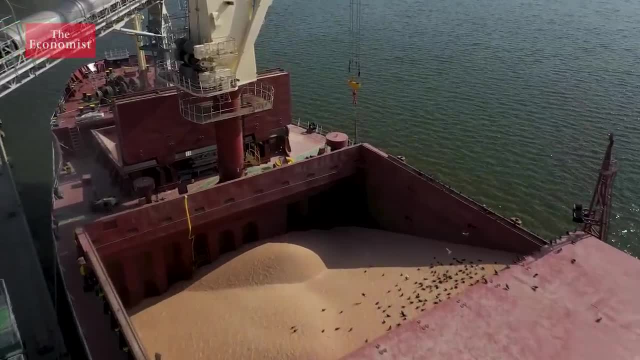 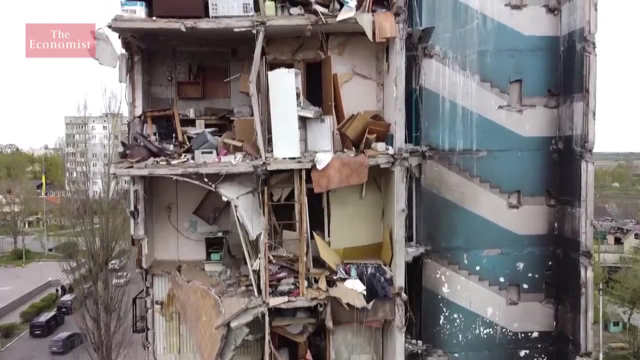 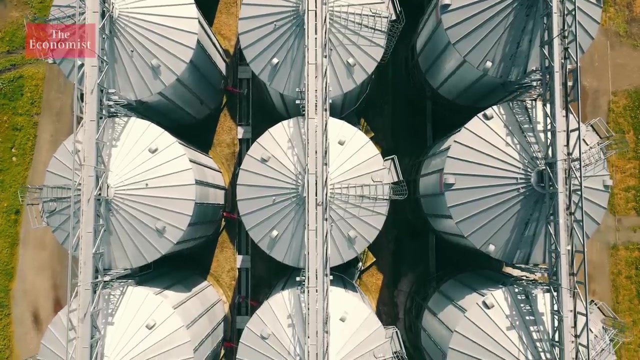 is to get Ukraine's exports back to the global market. International negotiations have been trying to do just that. But even with a deal in place, longer-term weaknesses in the world's food system would remain, Which is why experts continue to warn about the prospects for a world 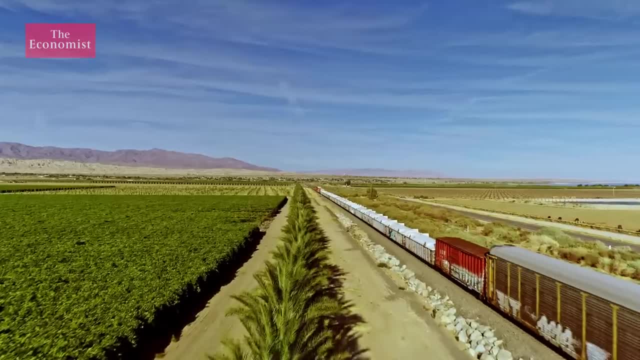 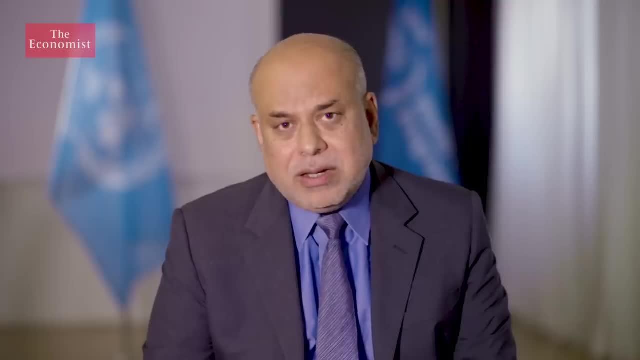 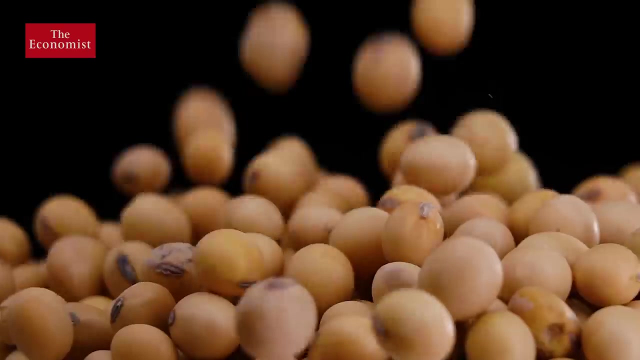 that remains too dependent on too few countries for its food. Less than 10 countries count for around 90% of our exports for key commodities like wheat, like corn, like rice, like soya beans. So when there is a shock in any one of these countries, 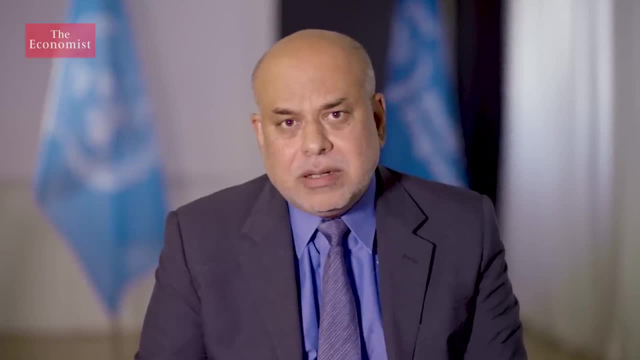 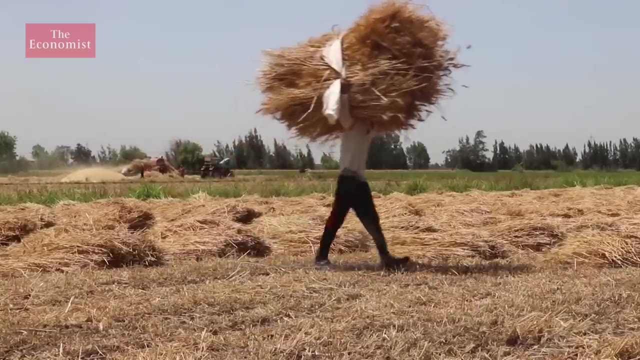 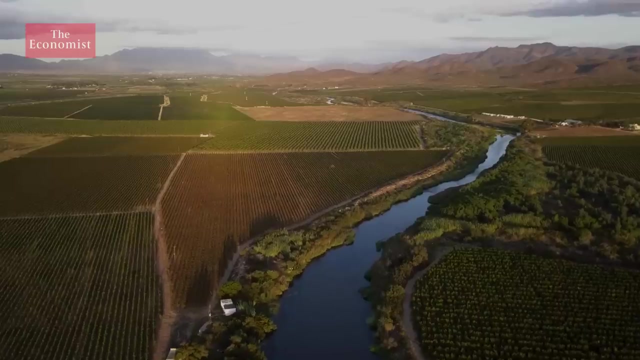 whether it be climate, whether it be conflict, you see the consequences of that across the world. Some countries are trying to insulate themselves from these shocks by becoming more self-sufficient. It's an attractive idea, And this year the World Bank announced that it's making $30 billion.